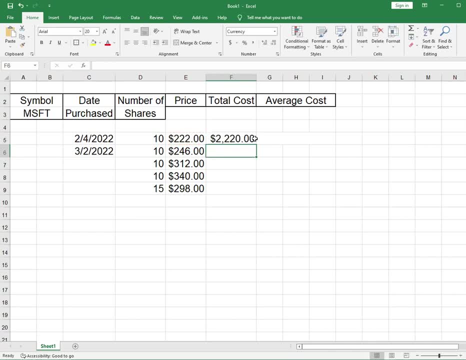 price here and we'll click enter. So our total cost for our first buy was $2,220.. Now we can grab this and we can run this down and that'll fill in the rest of our purchases. Why don't we center that? That's a little bit distracting. There we go. So if we use 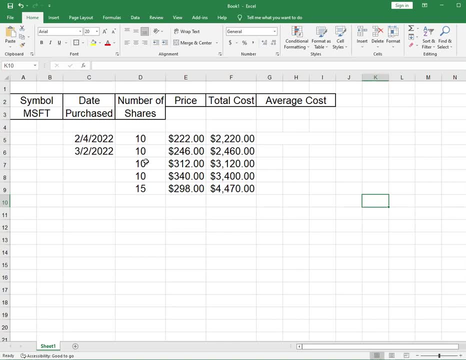 the auto-sum here. We can just drag this down and click the auto-sum. We'll center that We got 55 shares. We highlight those and do auto-sum again. We have a total cost of $15,670.. So our average cost we'll put up in here. 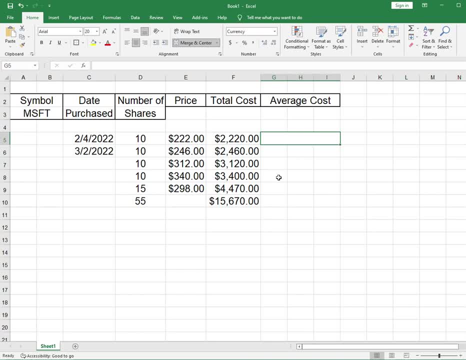 So this is a simple calculation and we can do this with Excel or we can do it with the calculator, But we just want to make sure that this is correct In Excel. Excel it says We just want to divide our total cost by our number of shares. 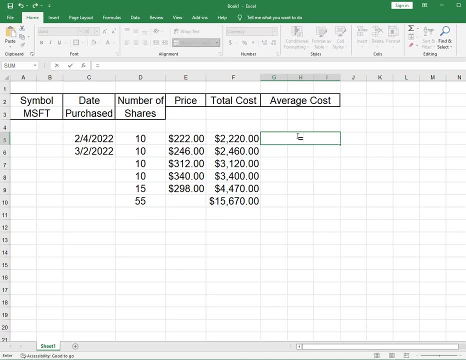 So, using Excel, we click in here, we'll type equals, we'll highlight this the divided by slash, which is down by the question mark, and we'll highlight 55, type enter. So our average cost per share is $284.91.. 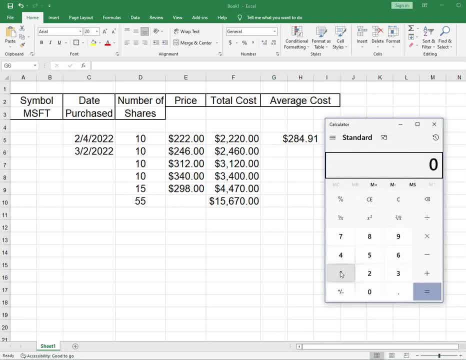 Now, if we did that with a calculator, it would be the same thing. we just type in: 15670 divided by 55 equals 284.90, and we'll round up to 91.. Okay, let's do one more example. 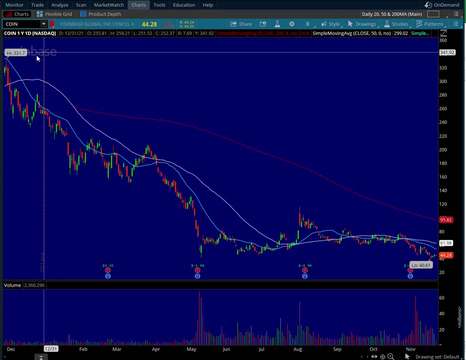 This time we'll use a simple coin and we'll show a bring up a chart here. Coin has really had a bad year from 331 down to 40. So we'll put in some- we'll just put in some more imaginary buys and we'll say we did. 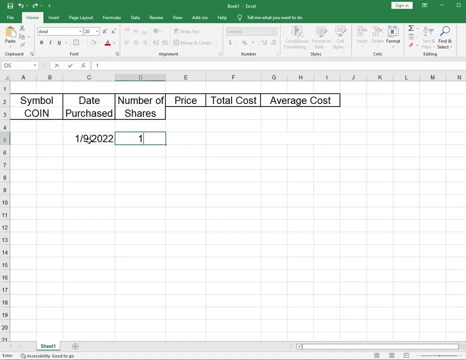 one in January and we did 15 shares at. we'll put in some cents, some odd numbers this time And, like I said, we really don't need these dates, but I'll just add some dates just to show here. And this time we did 35 shares, let's say 191.01..